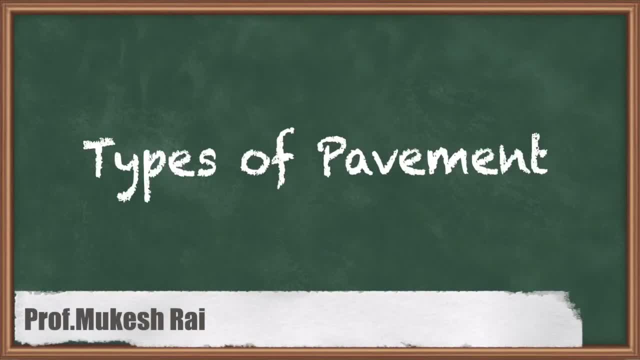 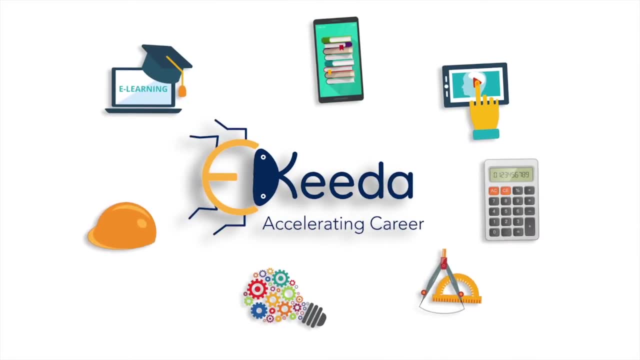 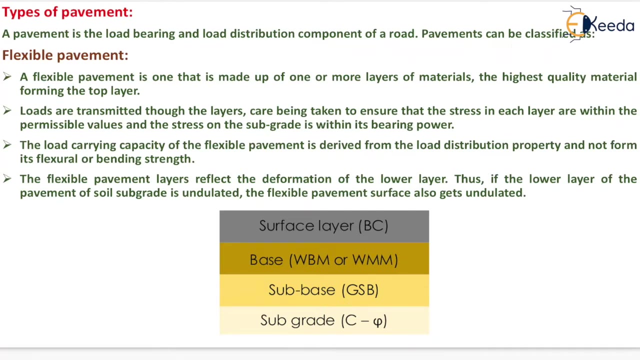 Hello students, today we are going to study types of pavement. A pavement is the load bearing and load distribution component of a road. Pavement can be classified as flexible pavement. Now, what do you mean by flexible pavement? A flexible pavement is one that is made up of one or more layers of materials. 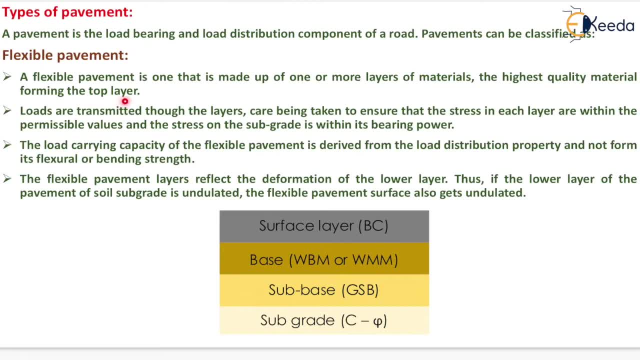 The highest quality material forming the top layer. Loads are transmitted through the layers, Care being taken to ensure that the stress in each layer are within the permissible values and the stress on the subgrade is within its bearing power. The load carrying capacity of the flexible pavement is derived from the load distribution property. 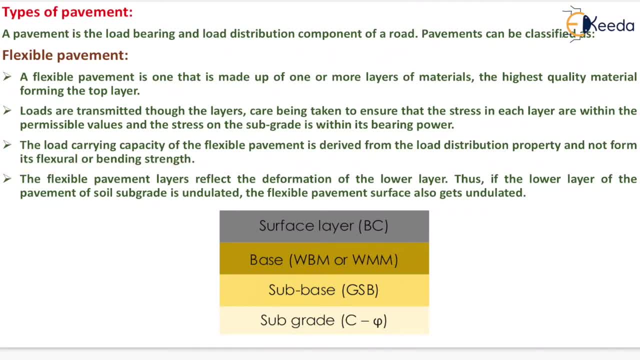 and not from its flexural or bending strength. The flexible pavement layers reflect the deformation of the lower layer. Thus, if the lower layer of the pavement of soil subgrade is undeleted, the flexible pavement surface also gets undeleted. Now, this is a particular cross section of a flexible pavement. 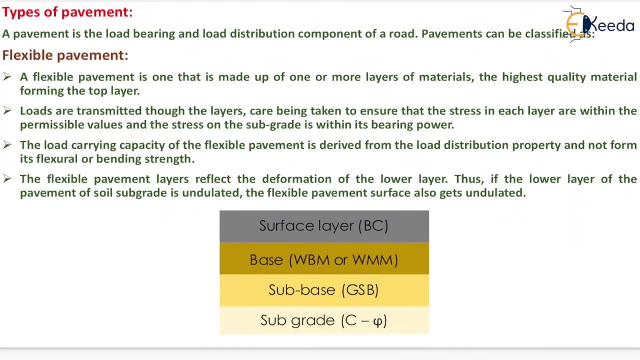 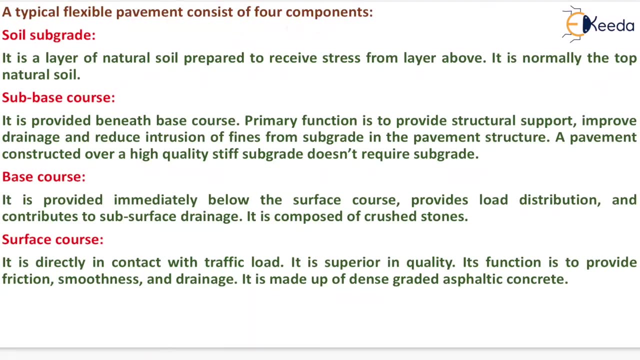 At the bottom, there will be a subgrade Above that subbase base course, and the last one, that is, the top course, is known as surface course or surface layer. Now, a typical flexible pavement consists of four components, which we had already seen. 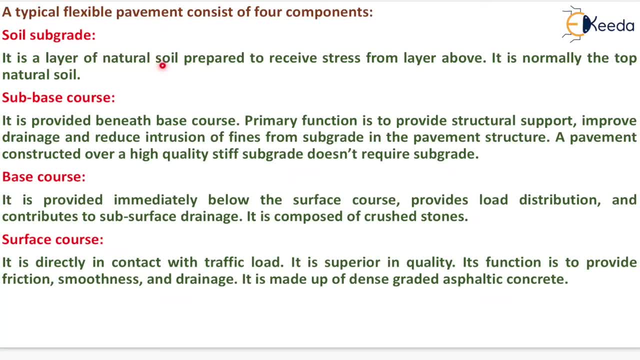 That is soil subgrade. It is a layer of natural soil prepared to receive stress from layer above. It is normally the top natural soil. Now the next one is the subbase course. It is provided beneath base course. the primary function is to provide structural support, improve drainage and reduce intrusion of fines from base course. 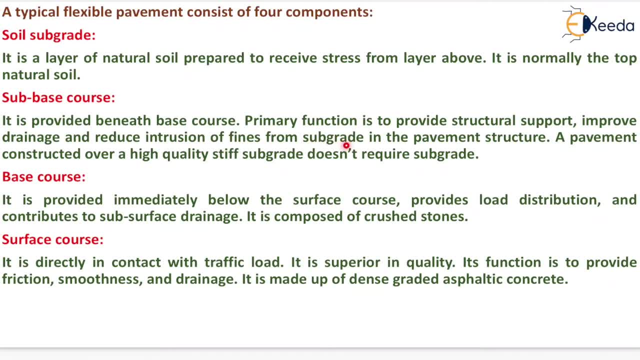 now. the next one is this subbase course. it is provided beneath the scores. primary function is to provide structural support, improve drainage and reduce intrusion of fines. subgrade in the pavement structure: A pavement constructed over a high quality stiff subgrade does not require subgrade. It means that when the pavement is constructed above the stiff subgrade, 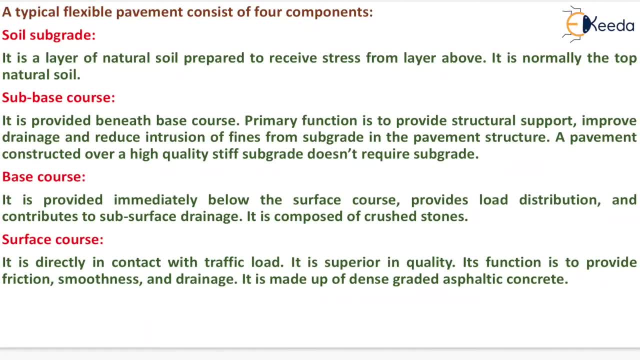 then it does not require any type of subgrade. Now the next is the base course. It is provided immediately below the surface course, provides load distribution and contributes to subsurface drainage. It is composed of crushed stones. Now the last course is the surface course, which 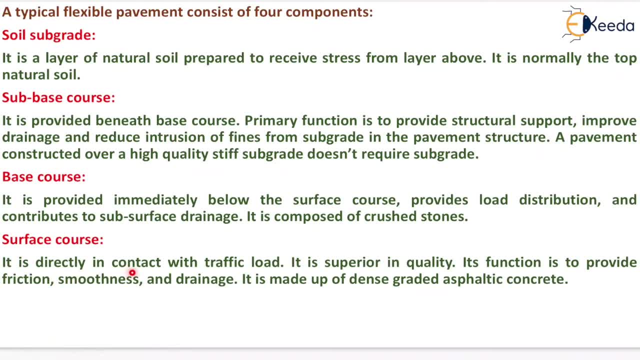 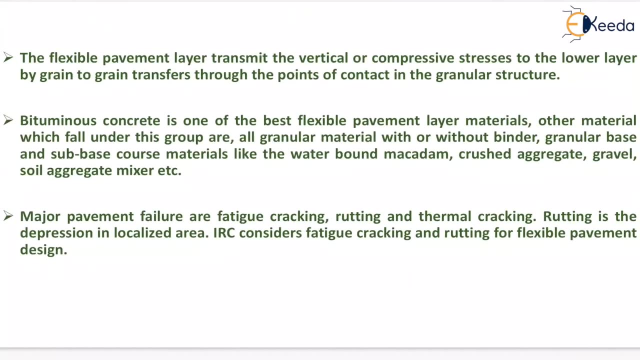 is also known as top course. It is directly in contact with traffic load. It is superior in quality. Its function is to provide friction, smoothness and drainage. It is made up of dense graded asphaltic concrete. The flexible pavement layer transmits the surface to the top course. It is made up of dense graded asphaltic concrete. 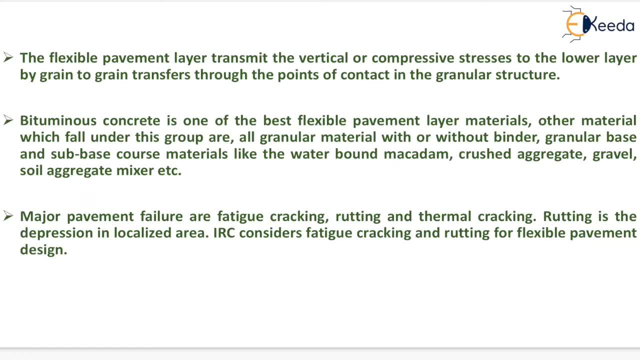 It is made up of dense graded asphaltic concrete. It is made up of dense graded asphaltic concrete. Subgrade the vertical or compressive stresses to the lower layer by grain to grain transfer through the points of contact in the granular structure. Bituminous concrete is one of the 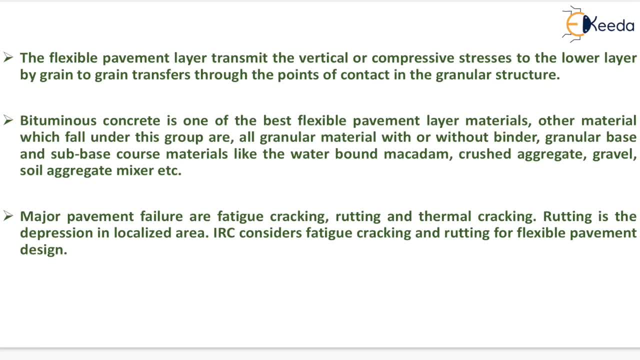 best flexible pavement layer materials. Other materials which fall under this group are all granular material, with or without binder, granular base and subbase course materials like the water bound mechanism, crushed aggregate, soil aggregate, mixer, etc. major pavement failure are fatigue cracking, rutting and thermal cracking. 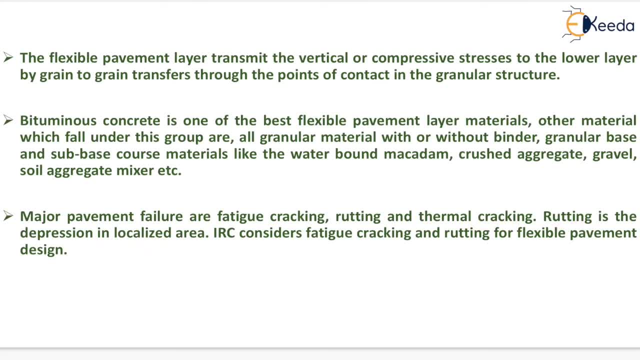 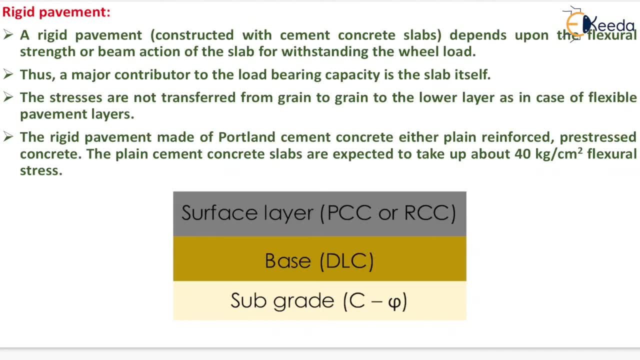 rutting is the depression in localized area. indian road congress considers fatigue cracking and rutting for flexible pavement design. now rigid pavement, which is our next type of pavement. a rigid pavement constructed with cement concrete slabs depends upon the flexural strength or beam action of the slab for withstanding the wheel load, thus a major contributor to the load bearing. 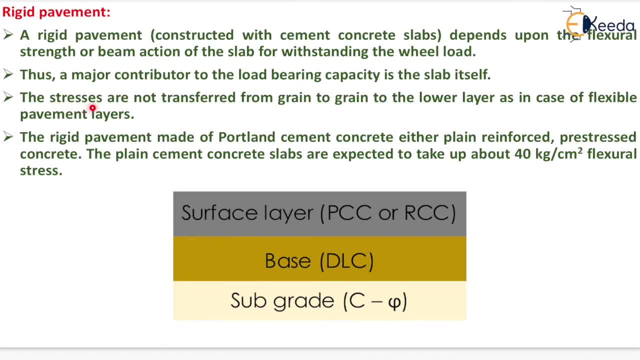 capacity is the slab itself. the stresses are not transferred from grain to grain to the lower layer, as in the case of flexible pavement layers. the rigid pavement made of portland cement concrete, either plain reinforced pre-stressed concrete. the plain cement concrete slabs are expected to take up. 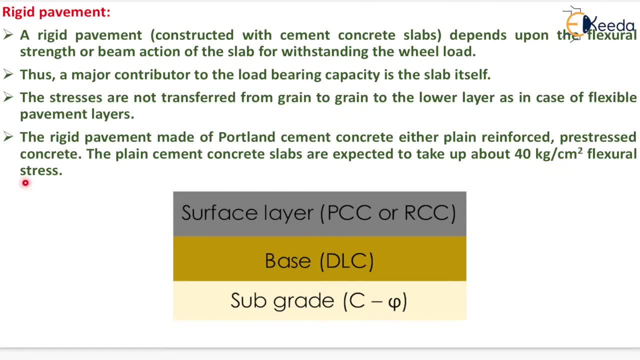 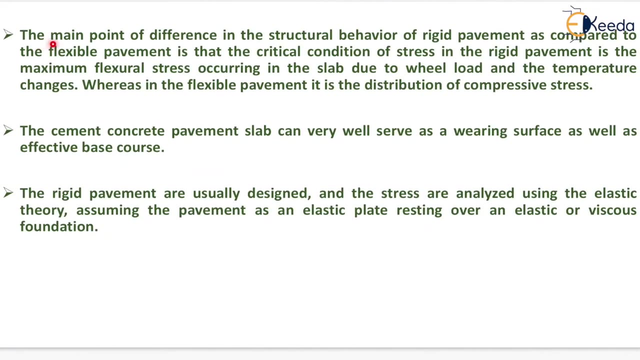 about 40 kg per centimeter square flexural stress. now this is a particular cross section of a rigid pavement. at the bottom there will be a subgrade above that base course. and the last one is surface layer or surface course, the main point of difference in the structural behavior of rigid. 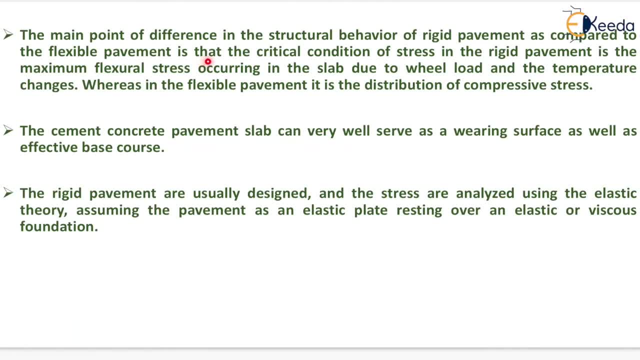 pavement as compared to the flexible pavement is that the critical condition of stress in the rigid pavement is the maximum flexural stress occurring in the slab due to wheel load and the temperature changes, whereas in the flexible pavement it is the distribution of compressive stress. the cement concrete pavement slab. 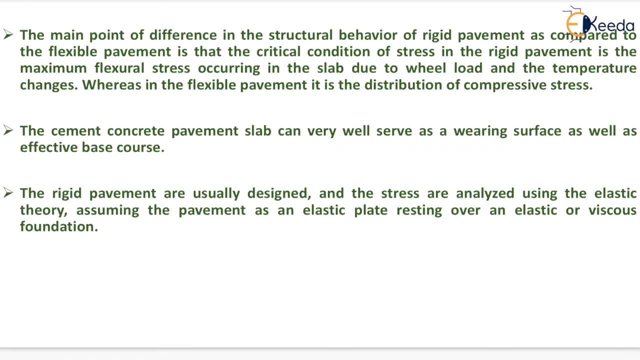 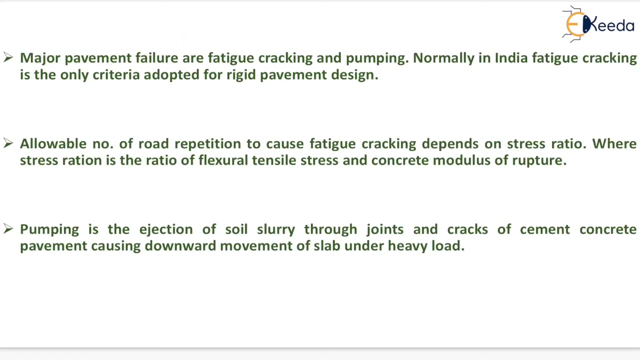 can vary. well serve as a wearing surface as well as effective base course. the rigid pavement are usually designed and the stress are analyzed using the elastic theory, assuming the pavement as an elastic plate resting over an elastic or viscous foundation. major pavement failures are fatigue cracking and pumping. normally in india fatigue cracking. 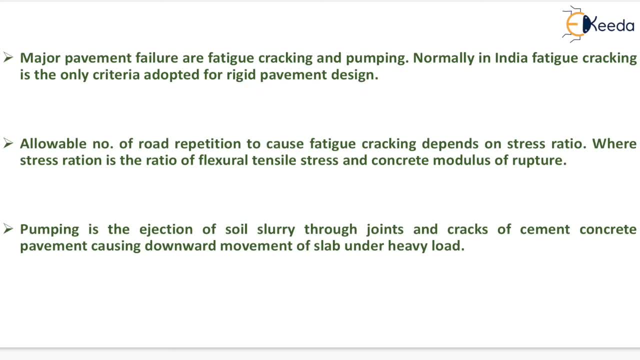 is the only criteria adopted for rigid pavement design. allowable number of load repetition to cause fatigue cracking depends on stress ratio, where stress ratio is the ratio of flexural tensile stress and concrete modulus of rupture. pumping is the ejection of soil flurry through joints and cracks of cement concrete pavement, causing downward movement of slab under heavy load. 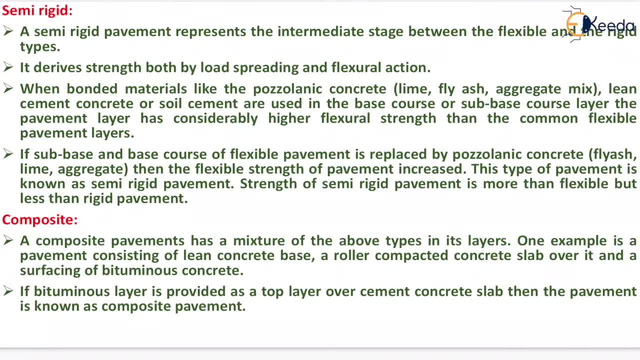 now. next type of pavement is semi-rigid pavement. a semi-rigid pavement represents the intermediate stage between the flexible and the rigid type. it derives strength both by load spreading and flexural action when bonded materials like the pozzolanic concrete, that is, lime fly ash aggregate. 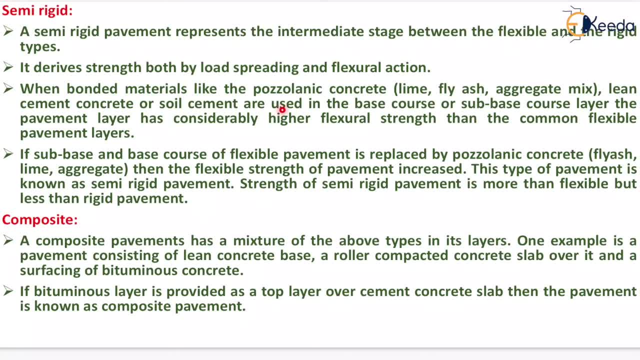 mix lean cement, concrete or soil cement are used in the base course or sub base course layer, the pavement layer has considerably higher flexural strength than the common flexible pavement layers. if sub base and base course of flexible pavement is replaced by pozzolanic concrete, that is fly ash.